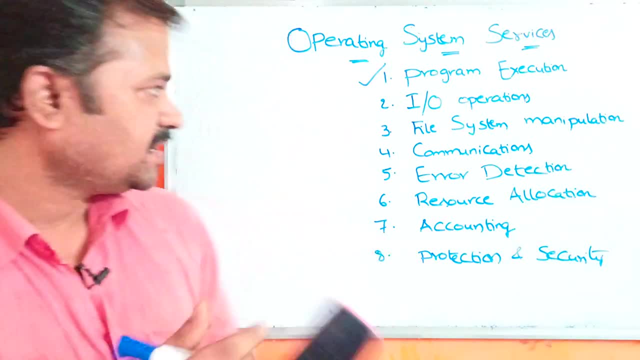 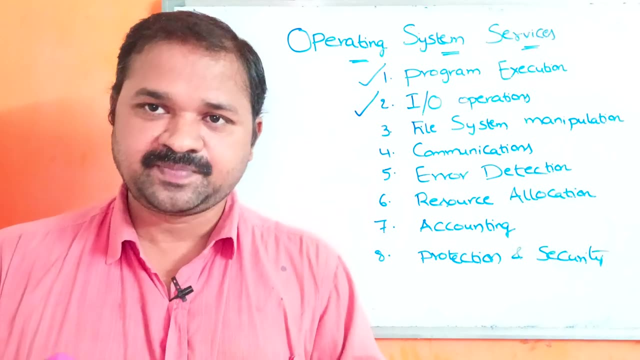 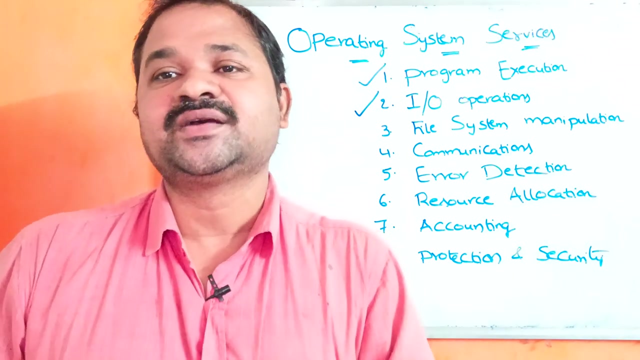 in order to do all these activities. Now let us see the next service, that is, Ivo operation- input output operation. When a program is in execution, the program may require an Ivo device or the program may require a file. It is the responsibility of the operating. 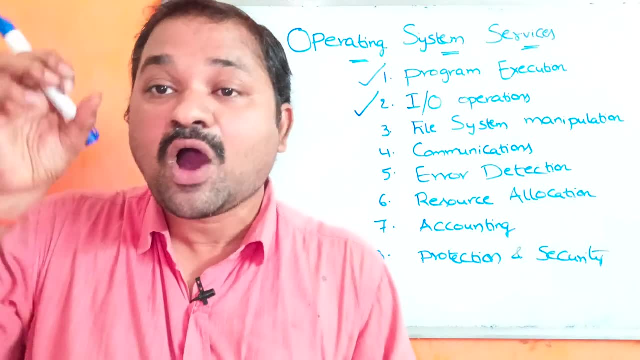 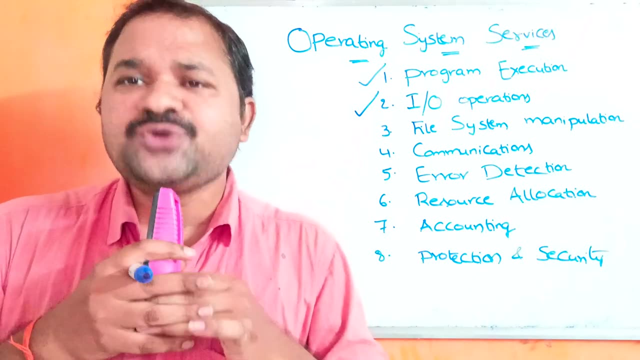 system to allocate the Ivo device to the hard disk. So when a program is in execution, the program may require an Ivo device or file to the corresponding program. Let us take the example of taking a printout. It is the duty of the operating system to allocate. 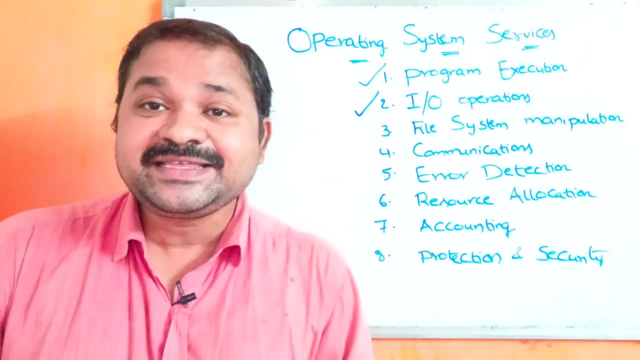 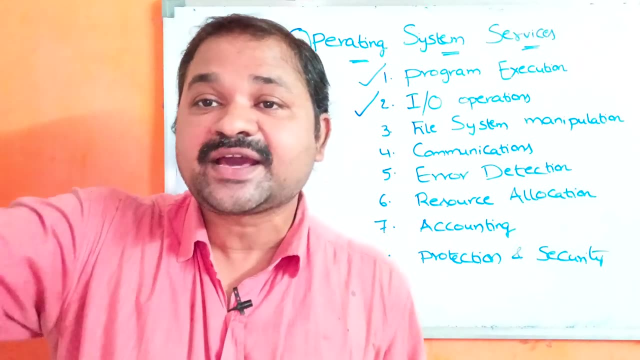 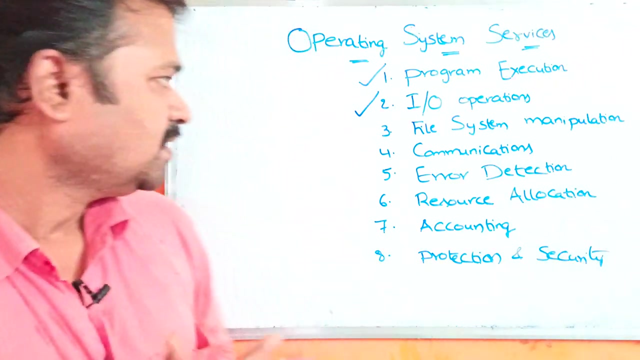 printer to the corresponding file. Let us take the example of scanning. It is the responsibility of the operating system to allocate scanner to the corresponding file. So Ivo operations will also be taken care by the operating system. Now let us see the next service, that is, Ivo operation When a program is in execution. 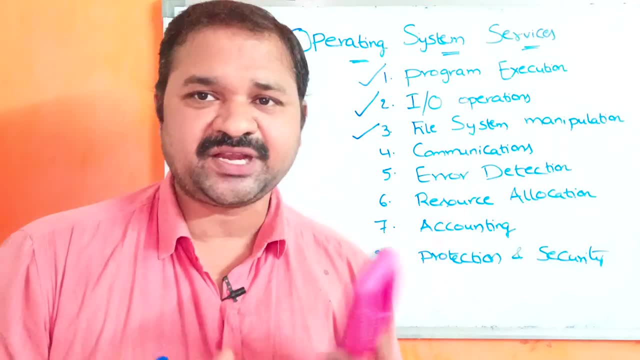 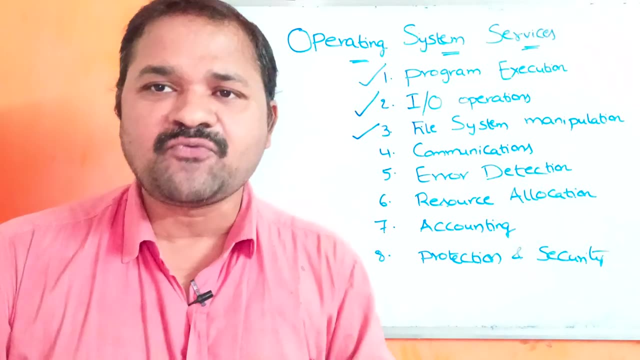 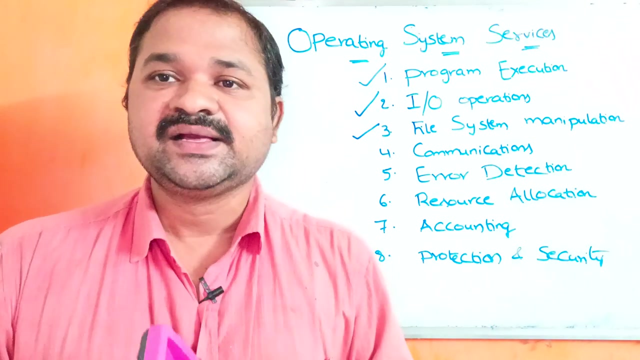 the next service, that is, file system manipulation. so what is a file system? if we want to organize a hundreds of files on lakhs of files, then we are using file system. so file system is a collection of directories. again, the directory may contain sub directories and directory may contains. 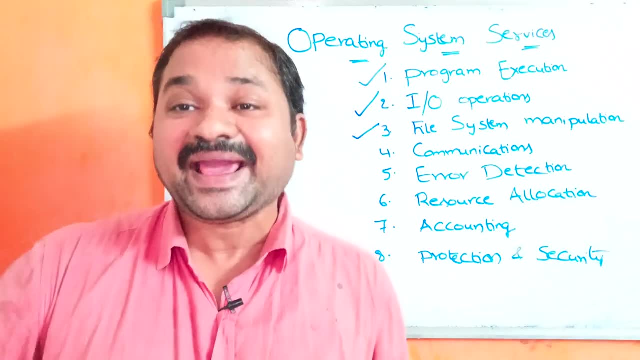 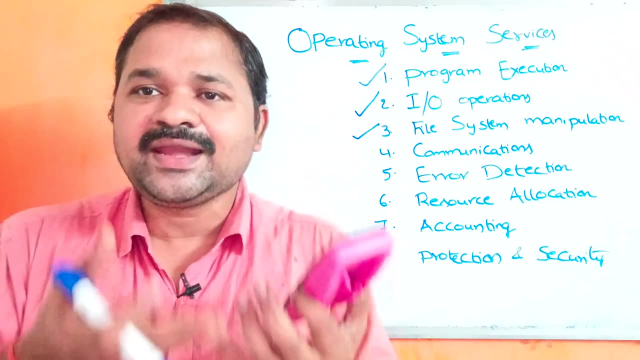 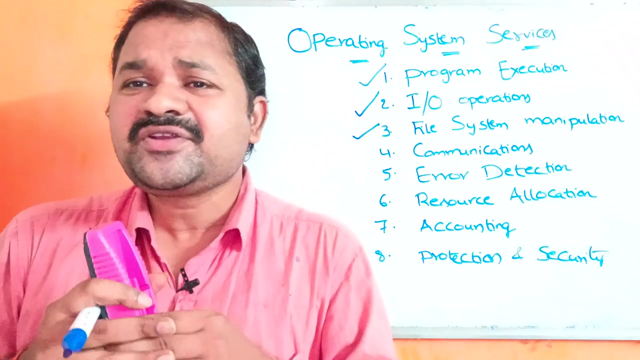 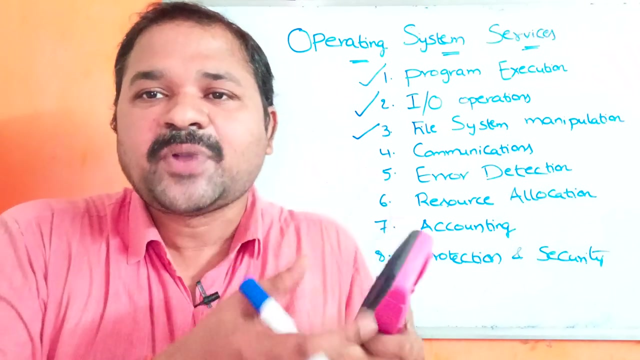 collection of files. every file contains some text. we can perform several operations on the files, such as creating a file, opening a file, performing the read operation, write operation, execute operation, appending operation. in order to do all these activities, we must need operating system. operating system will take care of performing all these operations. now let us see the next. 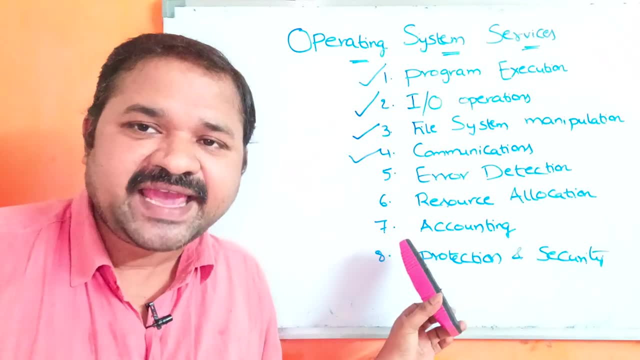 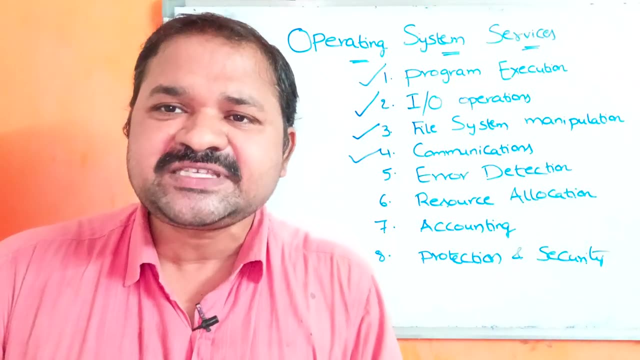 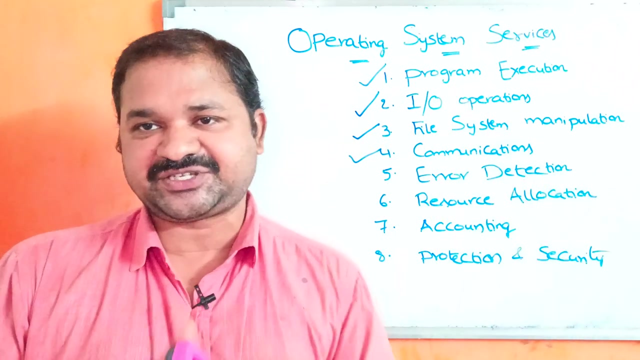 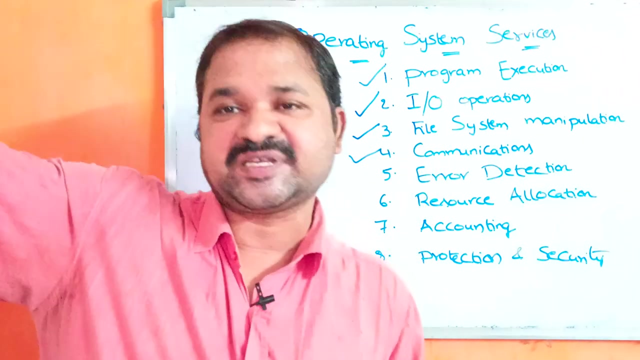 service, that is communication. one process can communicate with another process with the help of the operating system. only here those two processes may resides in the same computer, or those two processes may resides in different computers. so in some occasions one process may needs to exchange some information with other process. so that should be done with the help of the inter process communication inter. 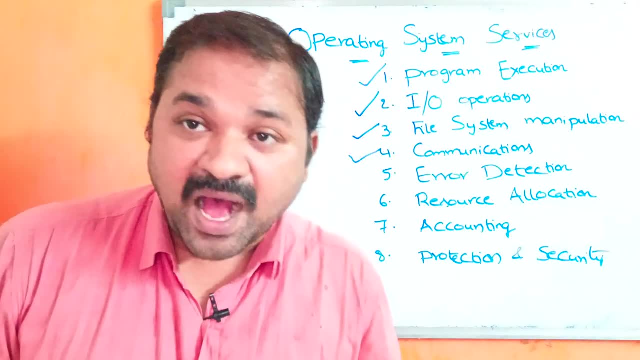 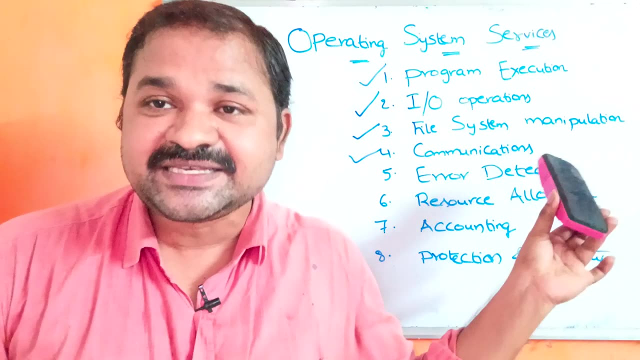 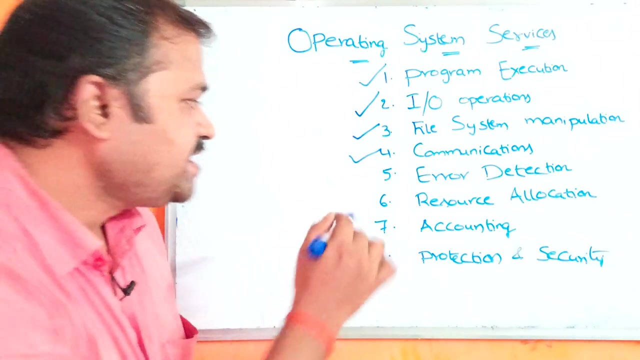 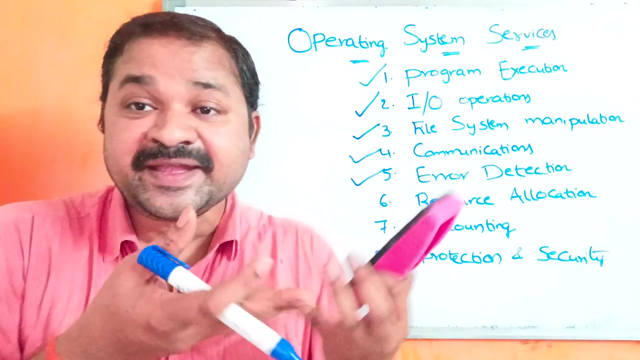 process communication is implemented with message passing and sharing of informations that we will see in inter process communication. So IPC, inter process communication, so that service will also take care by the operating system. now let us see the next service. that is error detection. so every time, every time operating system will detects, will monitor whether there are any errors or not. 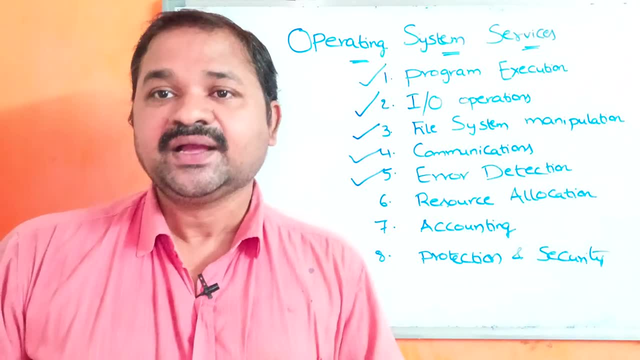 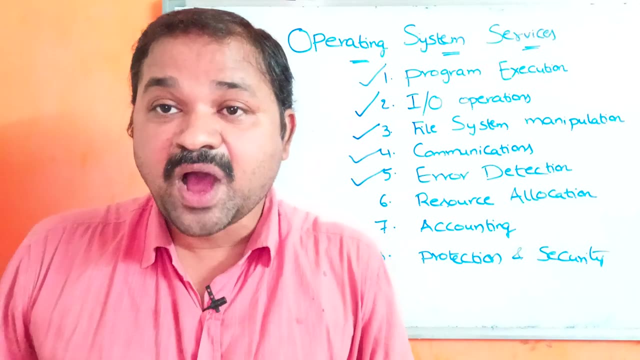 if there is any errors in the corresponding resource or not. it checks whether there is any error in the CPU or it checks whether is there is any problem with our mouse keyboard computer around the device, like Minitank or Lucid dei keyboard. so it is the responsibility of the operating system to detect errors in 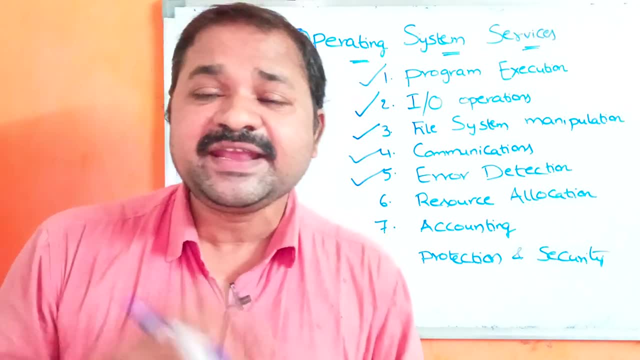 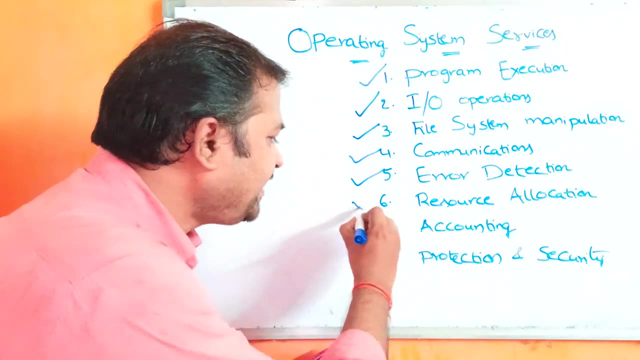 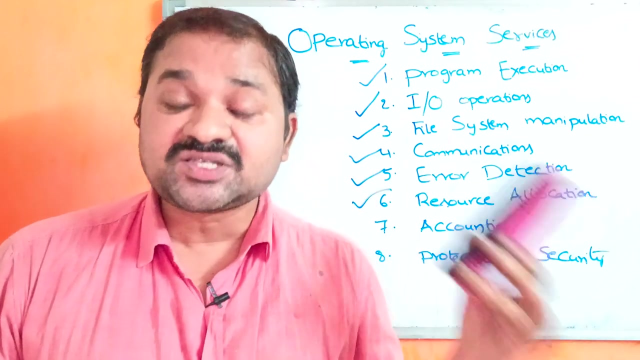 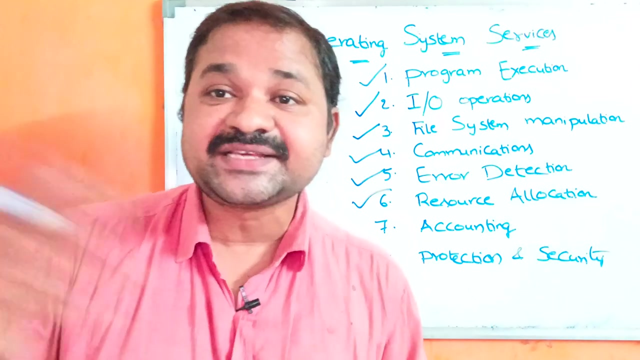 hardware devices and software devices. if there are any errors, then operating system will takes the appropriate action. now let us see the next service of the operating system, that is, resource allocation. we have several resources, such as hardware resources. under software resources we have CPU- it is a resource. main memory. RAM- it is a resource. hard disk- secondary memory it. 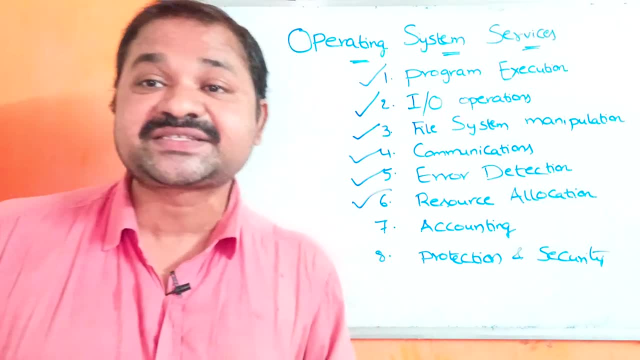 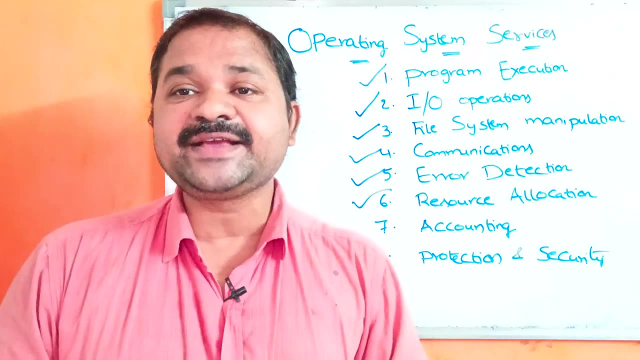 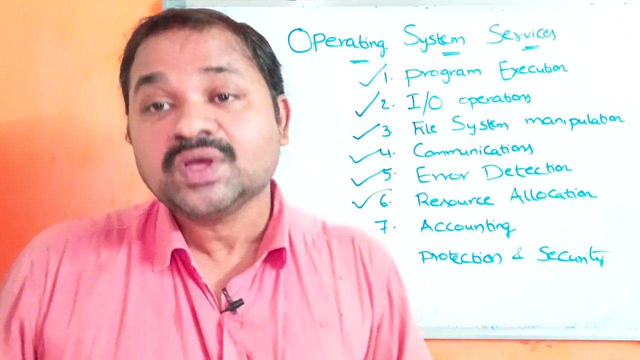 is a resource and software resources such as files. operating system will allocate all these resources to the program. it is the duty of the operating system to manage the process, to manage the memory, to manage the disk, to manage the Ivo, if we take a program execution. so after saving the program, what will? 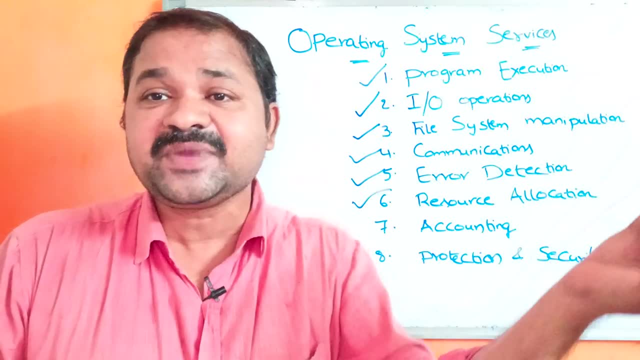 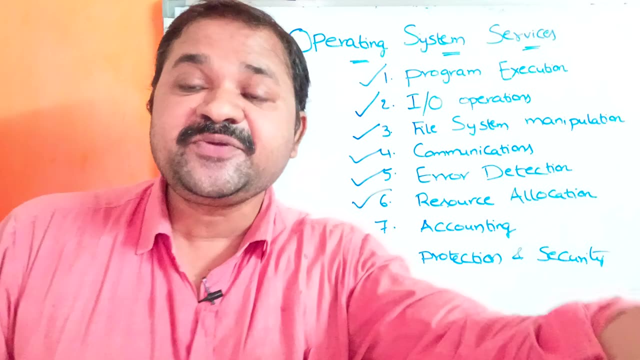 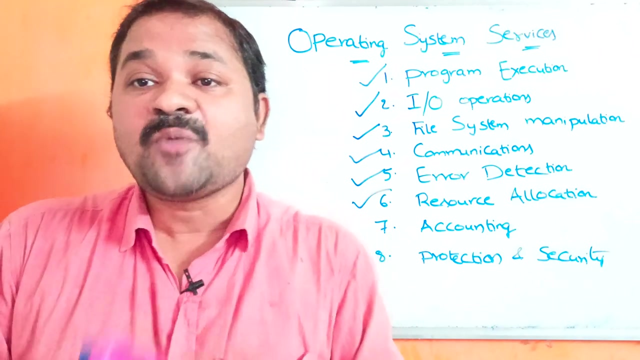 happen. the program will be saved in the hard disk, the it will be taken by the operating system only. so during execution, operating system allocates CPU to the program, so CPU starts executing the program. let us say, assume that that program requires some Ivo operations. so operating system. 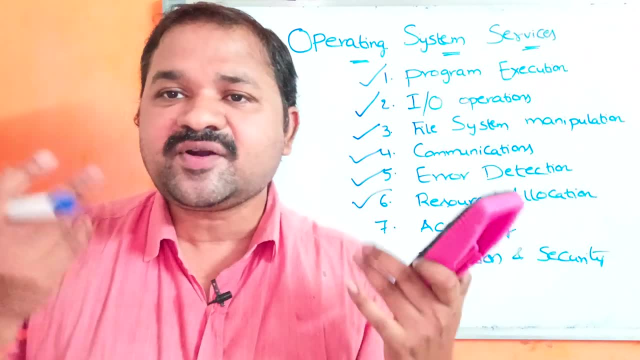 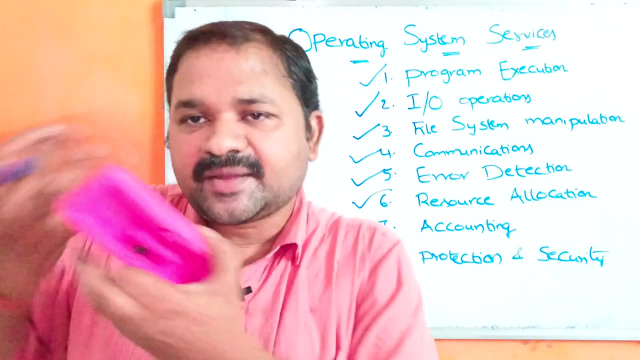 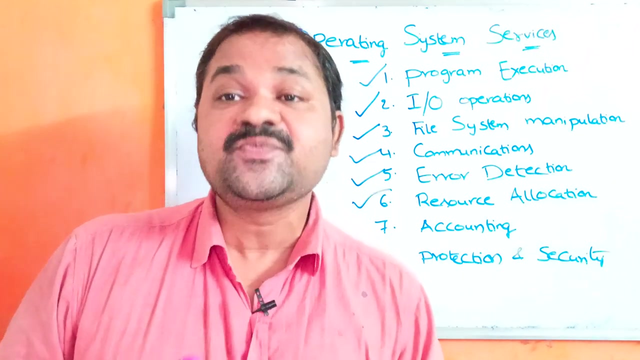 allocates CPU to some other program. why? because during Ivo operation there is no need of CPU, so operating system allocates the cut that corresponding Ivo device to the program. so all these resources management will be done by the operating system. only now let us see. 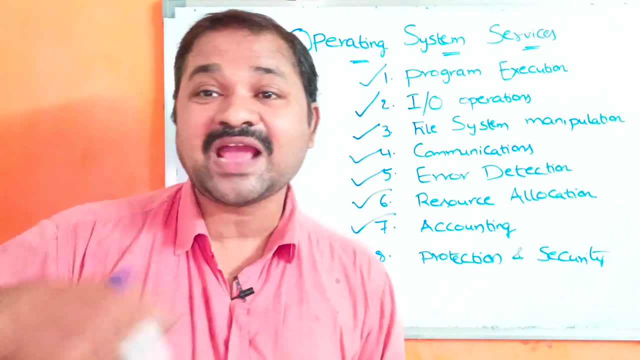 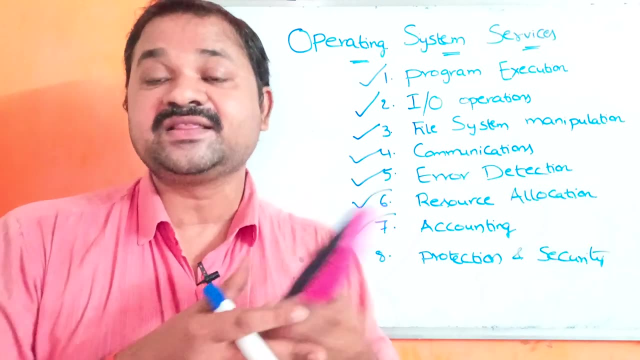 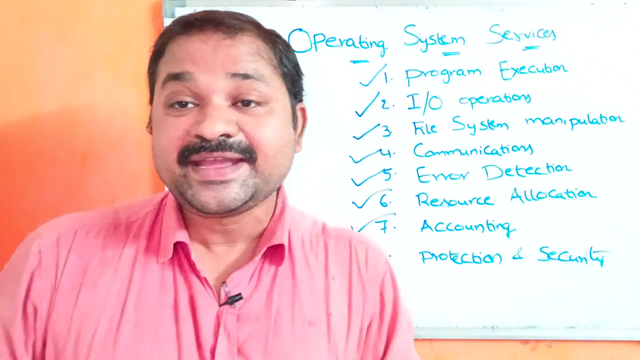 the next service, that is, accounting. let us assume that we have a network, so we know what is a network. network means a collection of computers so multiple persons can work in, can work with the computer. okay, multiple persons can work in that network, so operating system will monitors so which person uses which.